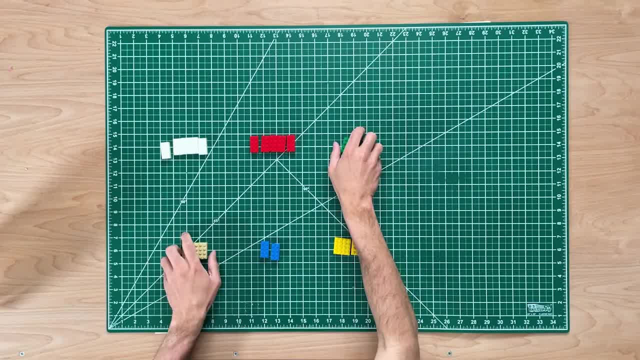 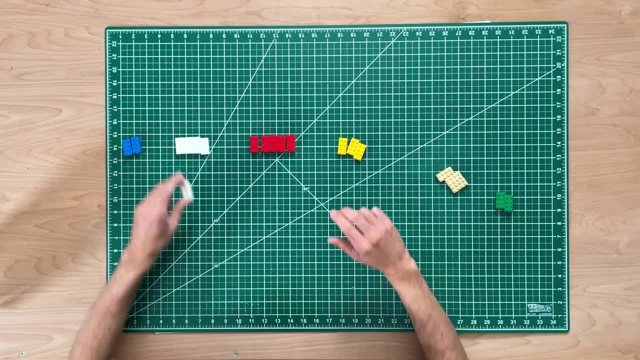 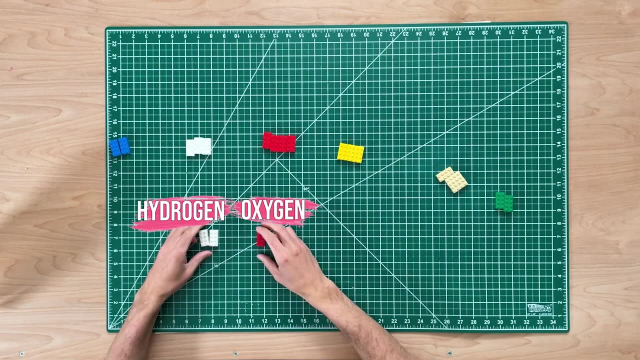 or chlorine. So today we're just going to focus on four of these elements. Now, if we take two atoms of hydrogen, so we're going to go one, two, okay, And now we're going to take one atom of oxygen And if we chemically combine the two- meaning we snap them together- 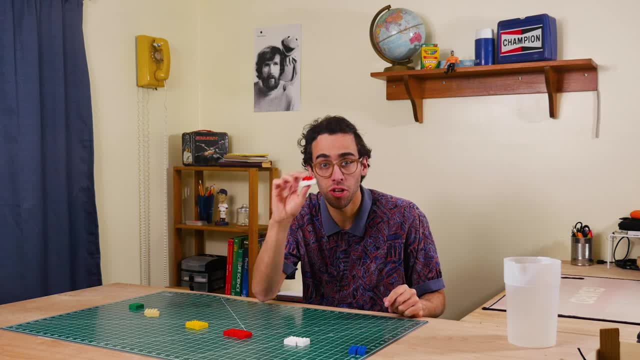 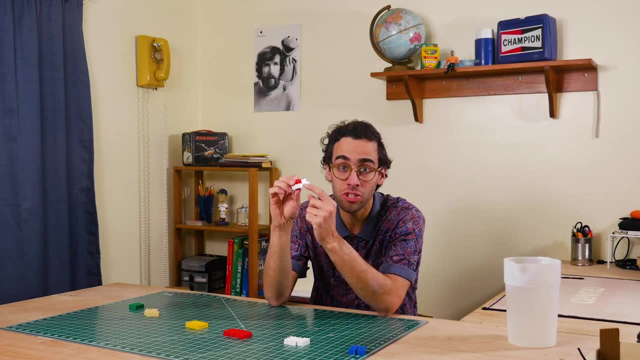 like this, we form an entirely new substance called a compound, And this compound is called H2O2.. H2O2.. Two hydrogens, one oxygen, Also known as water. All right, all right, let's make another one. 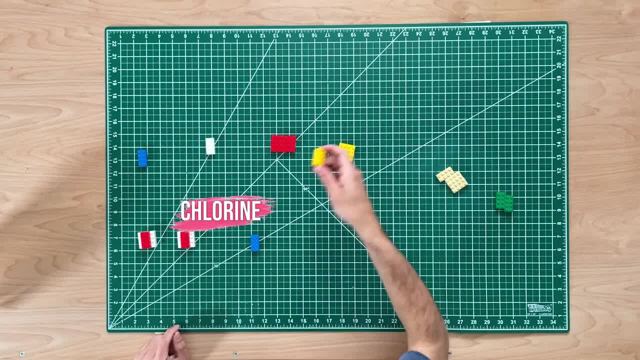 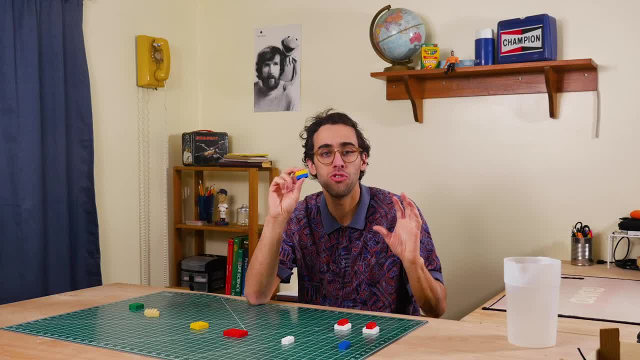 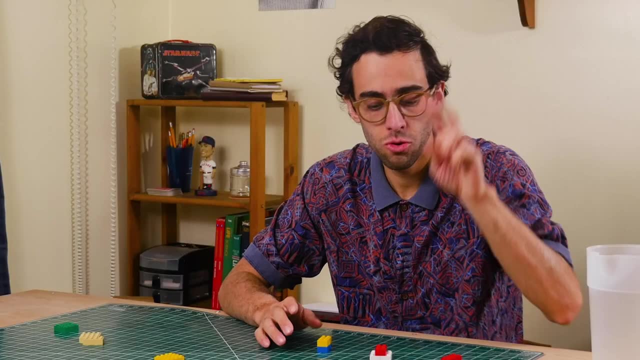 All right, so this time we'll take chlorine, a gas, and sodium, a metal- okay, And we will chemically combine them like this, And now we have an entirely new substance, a compound called sodium chloride or salt. So now we have two compounds, water and salt. What happens? 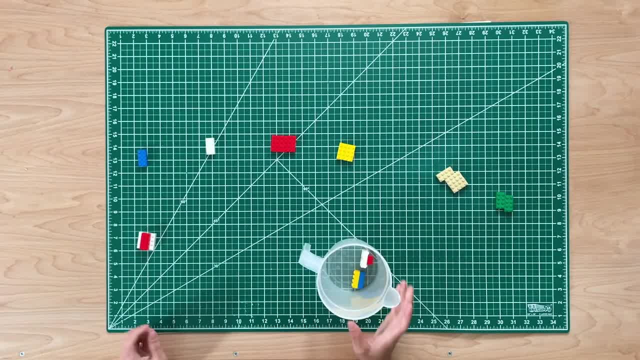 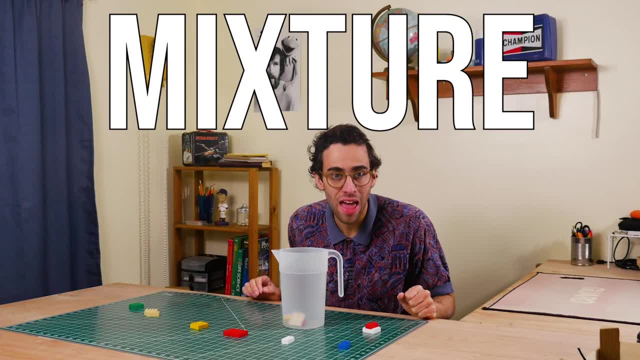 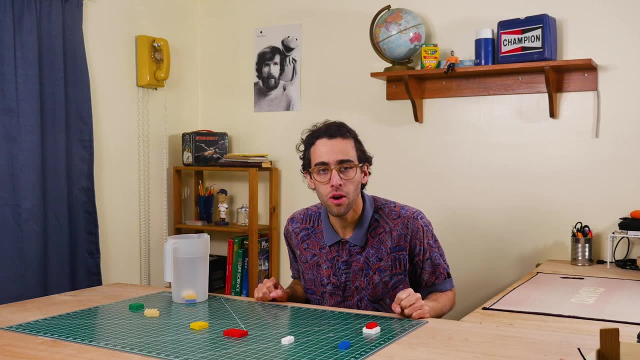 if we physically combine the two by putting them in a container, but don't snap them together, Well, we form a new substance, We form a mixture, And this mixture is salt water. Ooh, I smell the ocean, Mmm. So when two or more elements or compounds are physically combined, that means they form. 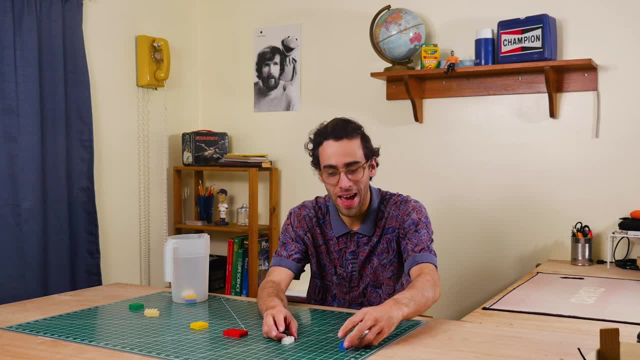 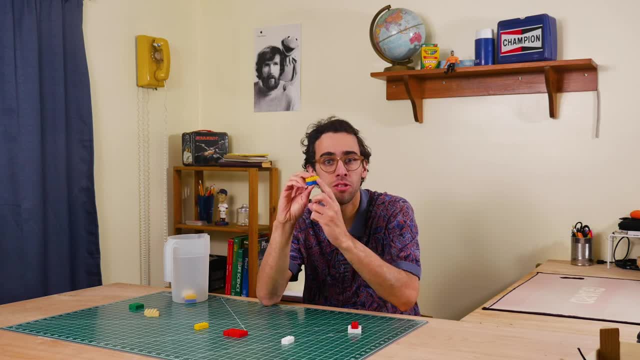 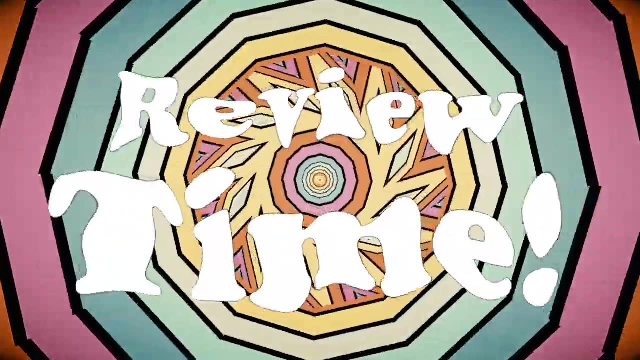 But aren't snapped together, Remember, because being snapped together means it forms a compound, And when they're near each other we'll call that a mixture. So, to review, I've created a worksheet so you or your students can try this on your own. 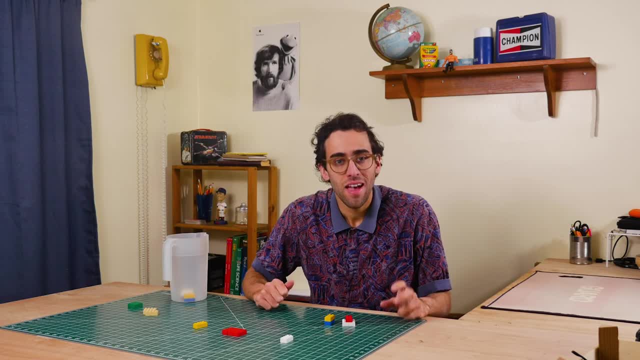 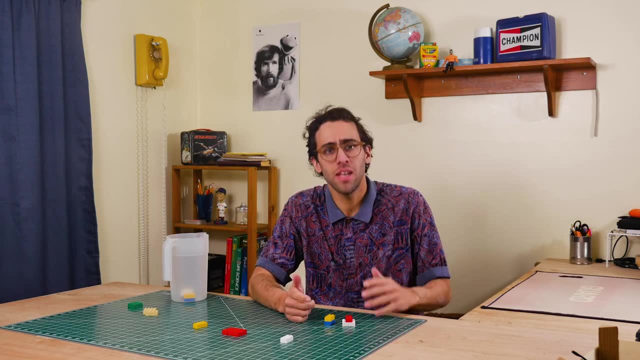 All you have to do is click the link below to download the worksheet, and you can begin building your own compounds and mixtures in Legos. Oh and, by the way, you don't need to use Legos: you can use knicks or magnet tiles. 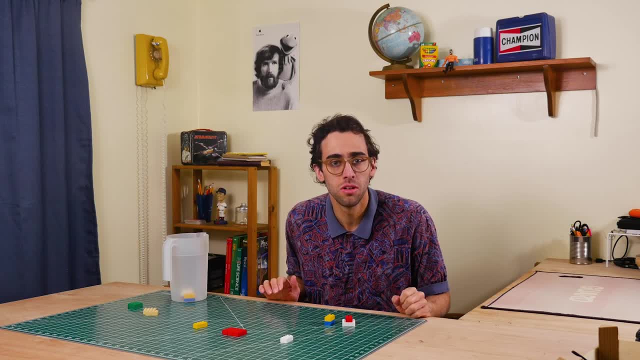 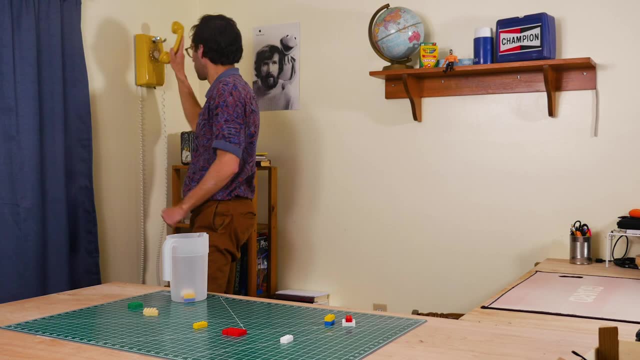 or whatever other colorful building blocks that you have access to. I better take this: Remember, be curious and ask questions. Yep, Okay, Quick, Awesome, Thanks, All right, bye.